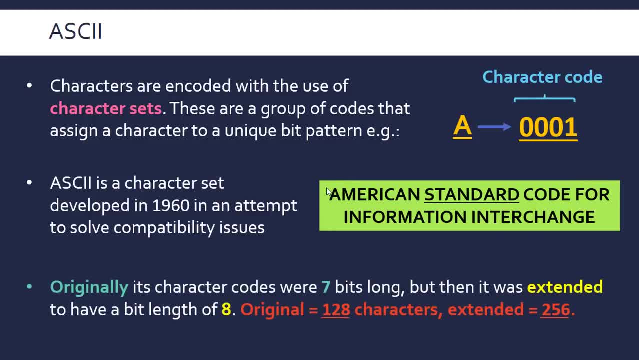 But I'll try and learn this acronym if you can. American is important because initially the codes were only seven bits long, but then it was extended to eight bits, So initial ASCII, or just ASCII, is seven bits long. Each character code is seven bits long, not four in this case. 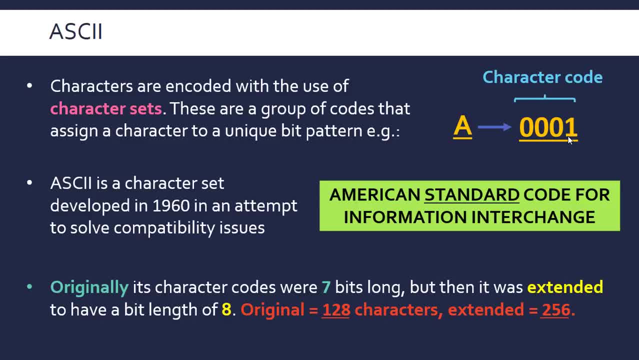 And then extended. ASCII has an eight bit long character code for each character And the issue is: with seven bits you only get 128 possible characters. Two to the power of seven is 128. So you only have 128 unique characters you can represent. And even with extended, it's not that much more. You only have 256 characters And that's not really enough for all possible characters you might use. It's enough for just your American language and various other symbols, But for other languages, like if you want to add Mandarin or an acrylic system, there's not enough space to store them. 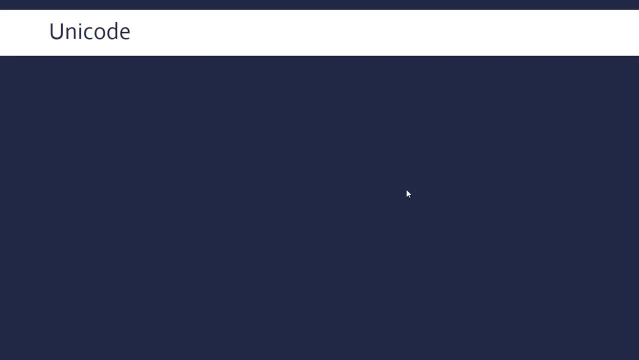 So this couldn't really be a worldwide system. So, because ASCII was unable to represent all possible characters, a new character set called Unicode was developed, And Unicode is much larger. So ASCII, is worth saying, is a subset of Unicode. So basically they share character codes up to 127. 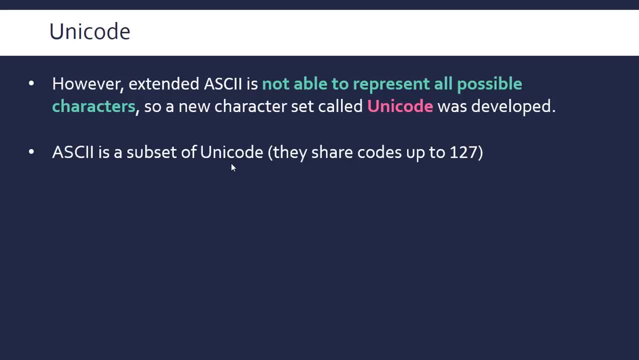 So all the character codes for ASCII are the same for Unicode It's just. Unicode goes way beyond that, And Unicode is not as simple as ASCII. It used initially 16 bits for each character, But this has since been expanded and it's a lot more complicated. So technology has developed. It has a much cleverer way of doing things, which we can't really go into, And there are loads of different standards that get released periodically, So it's not as simple as just saying there are seven bits in ASCII. 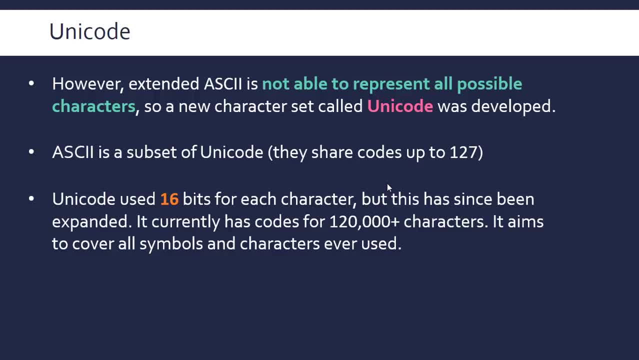 So, assuming it does use 16 bits, which it doesn't necessarily or doesn't anymore- This gives us 65, over 65,000 combinations, which is a drastic increase in ASCII. So that's the first thing, So that's the second thing. 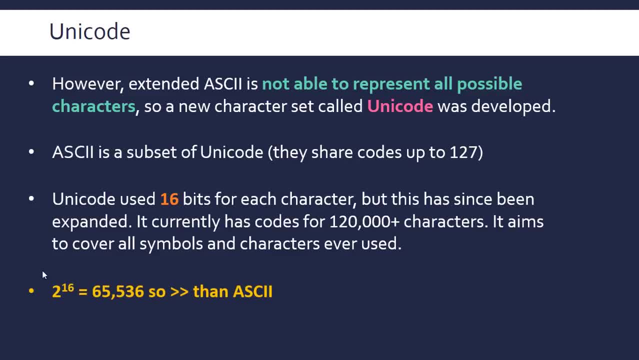 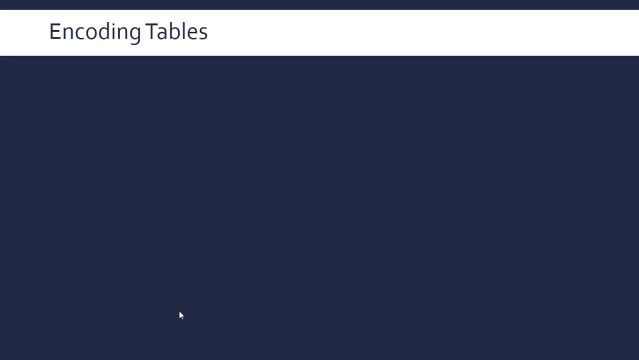 So the third thing is that it's a bit more complex, So it's a bit more complex. It's a bit more complex, So it's a bit more complex, Which is a drastic increase in what ASCII could. So you can kind of think of the character sets as just big tables. 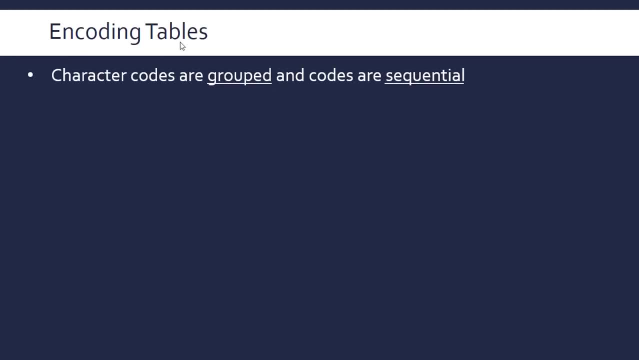 Big encoding tables, ie associating a code with a character. Big encoding tables: ie associating a code with a character, And it's important to realise that the character codes are grouped and the codes are sequential, And what this means is so they're grouped in terms of 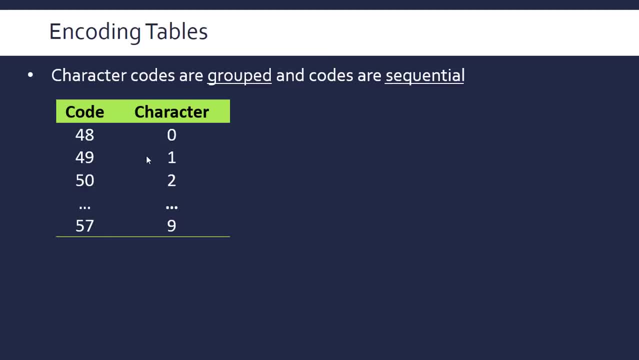 numbers and control symbols and uppercase letters and lowercase letters, and the sequential means that the characters are kind of logically or the codes increase logically based on what the characters are. So if we write the codes in decimal letters, of course in a computer they'd be the binary equivalent and they're also sometimes written in hexadecimal.